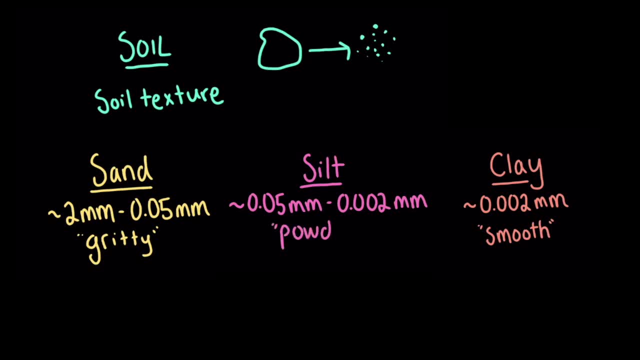 It's powdery, Powdery And it can be carried easily by wind and water. But soil is more complicated than just these three soil types. If you grabbed a handful of soil from outside your home, it would probably be a combination of all three soil types, along with some organic material. 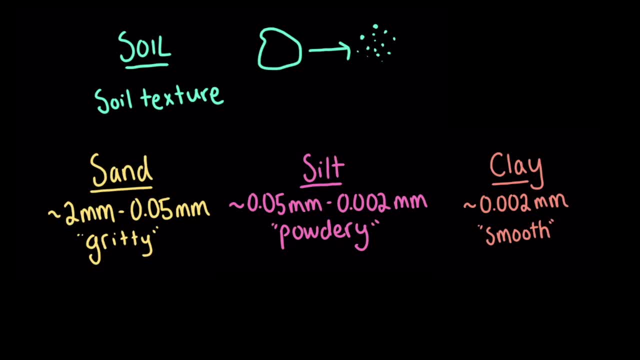 A soil's unique texture, that is, its combination of silt, sand and clay, affects how plants will grow, And so gardeners often want to know about their soil texture so they know what kinds of plants to grow in that area. 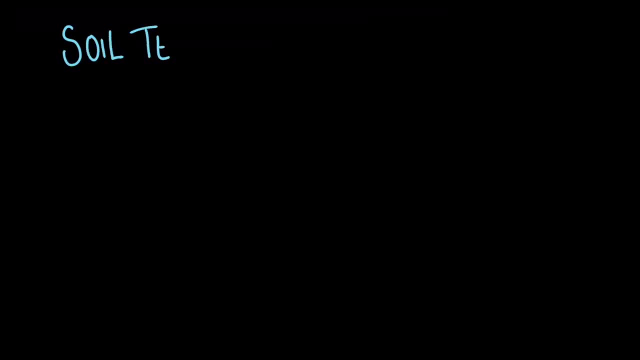 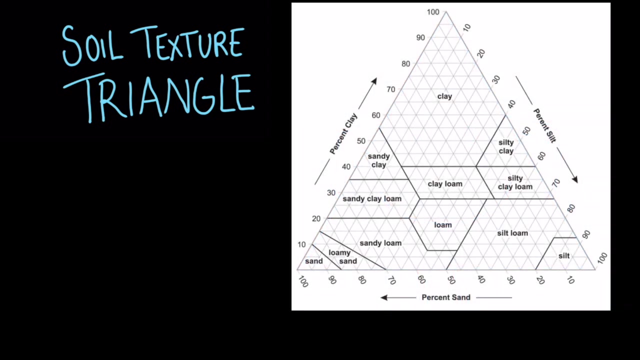 This is where a helpful diagram called the soil texture triangle comes in The soil texture triangle. The triangle allows us to place any soil sample into one of twelve different soil texture categories. The twelve different categories are broken up based on the percentage of silt, clay and sand in the soil. 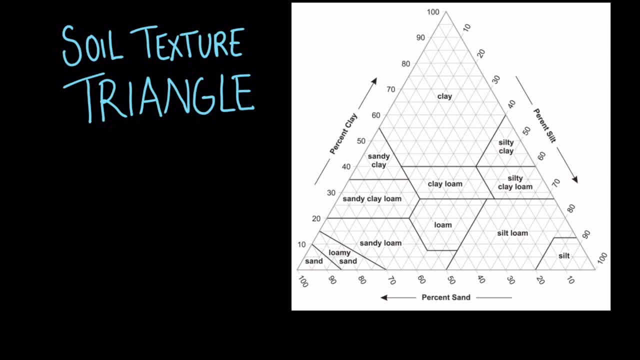 To see how this works, let's do an example. Let's say a gardener determined that her soil was 30% sand, 40% silt and 30% clay. So how can we figure out what kind of soil we have? 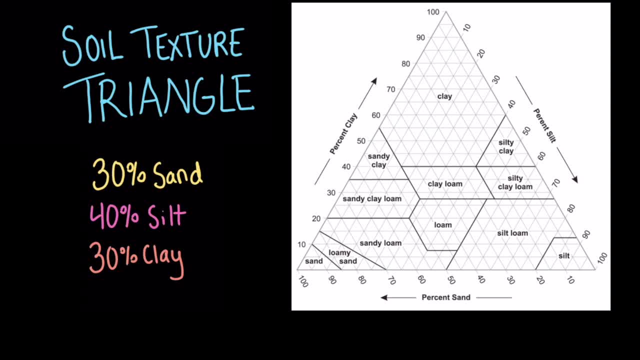 First, we need to pick a side of the triangle to start with. I'll start with sand. We know we have 30% sand, so we go along the side of the triangle until we find the 30% mark right here. 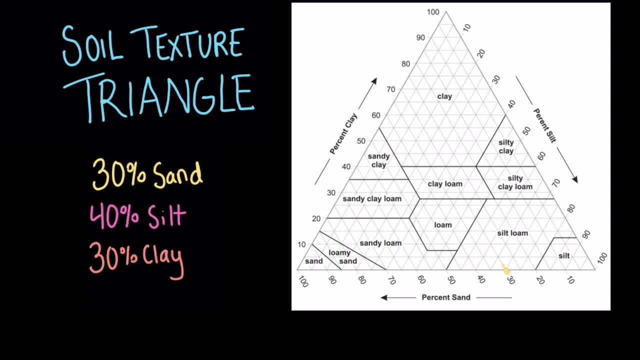 We want to draw a line from this point to the side of the triangle that this arrow is pointing to. The arrow is pointing towards the clay side, so we draw the line from the 30% sand mark through the triangle to the clay side. 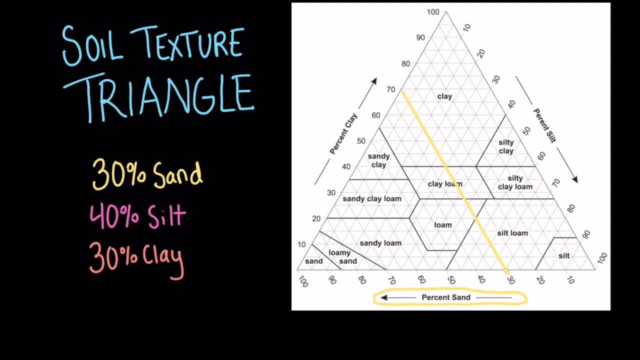 Like this, And by drawing this line, we already know that our soil sample will fall into a category along this line. So it could be silsloam, loam, clayloam or clay, But to figure out exactly where it is, let's draw another line. 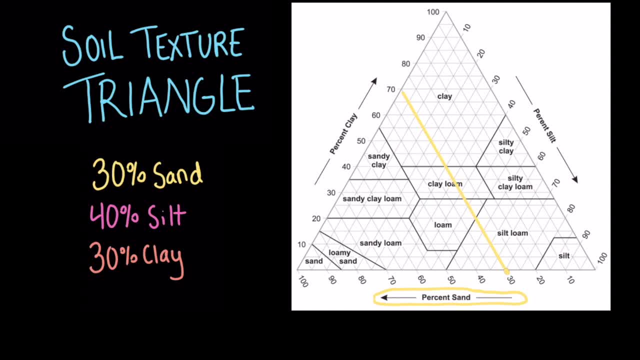 Let's do silt. The soil has 40% silt. We'll draw our line through the triangle towards the sand side because of this arrow. So again we do the same thing: We go along the percent silt line. 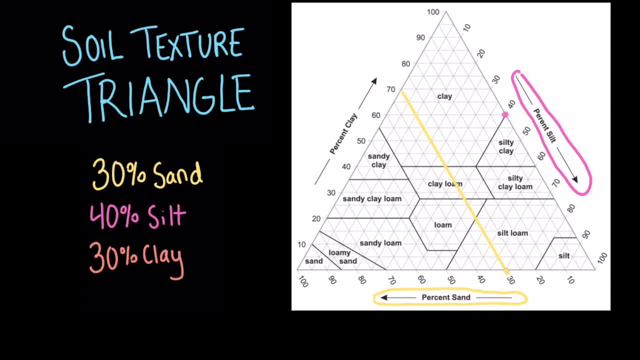 we find the 40% mark and we're going to draw a line from 40% to the other side of the triangle And you can see when we draw that line. these two lines intersect at the clayloam point. But to double check, let's draw a line from the 30% clay mark. 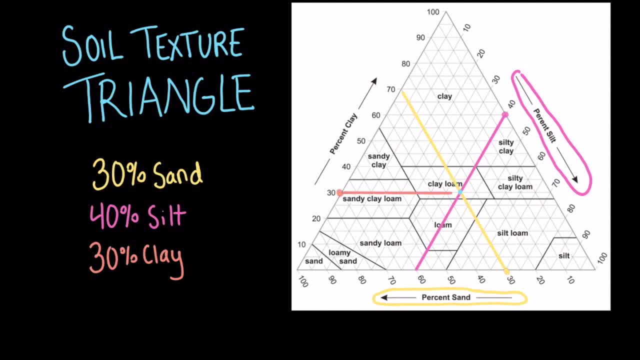 to the other side of the triangle like this. As you can see, these three lines all intersected at the same point right here in clayloam. So we know that we have clayloam. Notice that the percentage of clay, silts and sand all add up to a total of 100%. 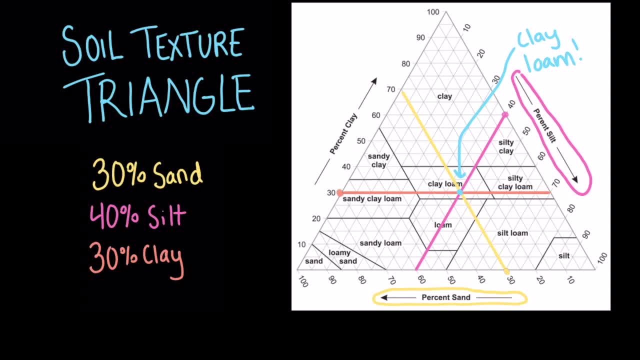 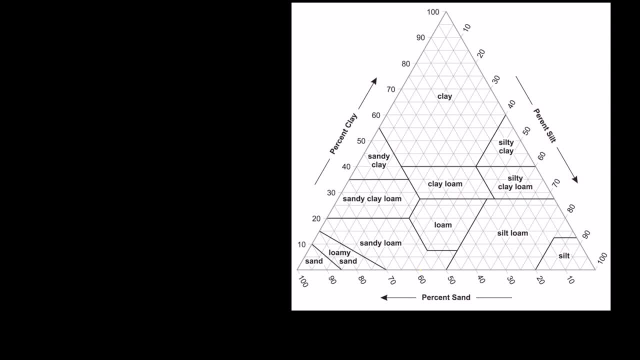 We could have picked any two of these lines, just two, to find our answer. We don't need to draw three lines every time. Let's do another example. Let's say: our gardener has another plot that contains 58% sand. 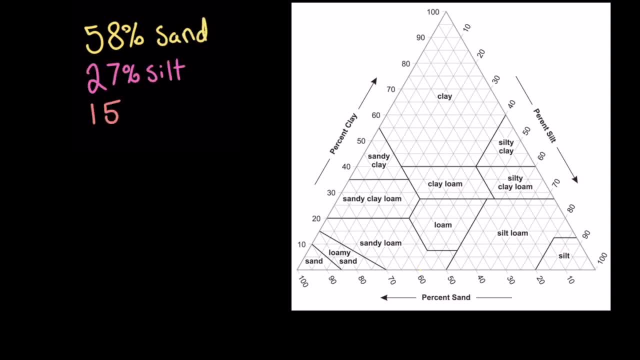 27% silts and 15% clay. So I'm going to go along the percent sand part and find 58%. so that's pretty close to 60. And I'm going to draw a line from 58% to the other side of the triangle. 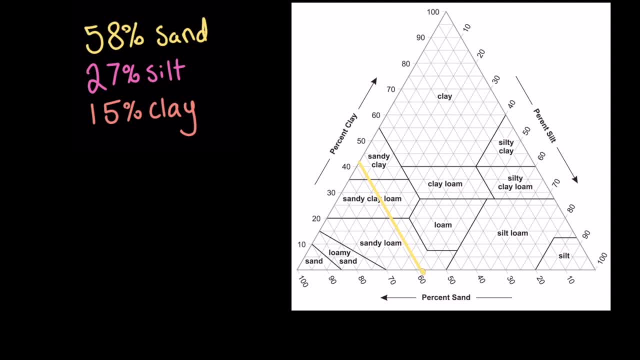 Sometimes the example question doesn't give us round numbers to work with, So when that's the case, I like to use a ruler or a straightedge just to make sure that my lines are in the correct spot. Next, I'm going to use the 15% clay. 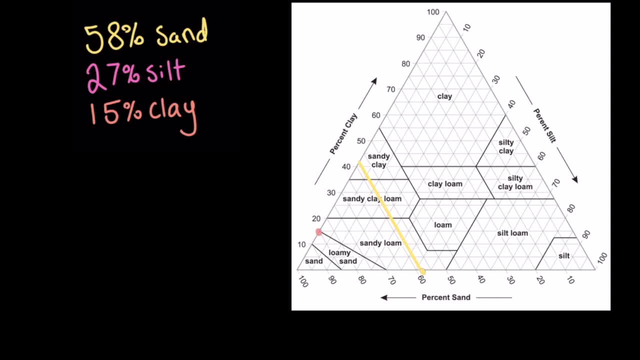 So I find the 15% clay mark and we draw a line from 15% to the other side of the triangle, following the direction of the lines within the triangle, And we can see that our two lines intersect at this point. So we have sandy loam. 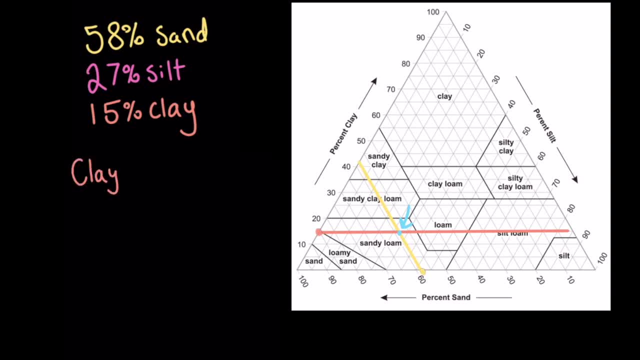 The gardener has these two plots, clayloam and sandy loam. So when the gardener looks at her two plots she might want to take into account the different kinds of soil. Certain kinds of plants do better in clay loam soil.